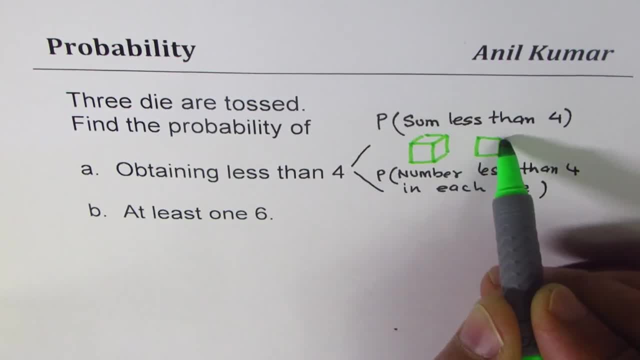 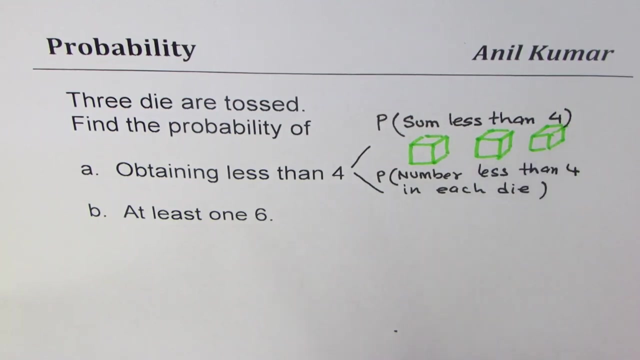 So our third digit is forty four. This is my three different dies. right, I need to calculate size. right, There is one option. All right, We looked at this, That's all. Let's solve some more. Let's do this. 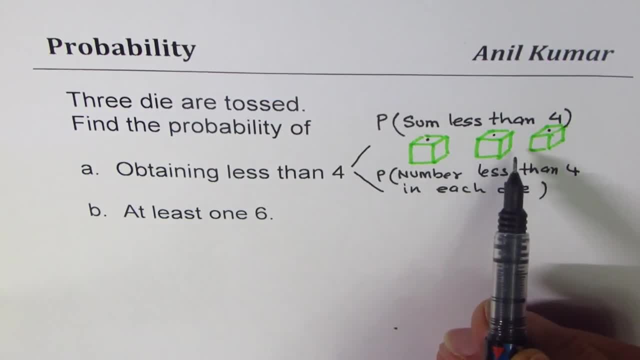 Okay, All right, Uh-huh, Okay, be less than four, right, and what are the total number of options? so the total number of options are: there are six phases. therefore, in case of three dies, total number of options will be six to the power of three, six to the power of. 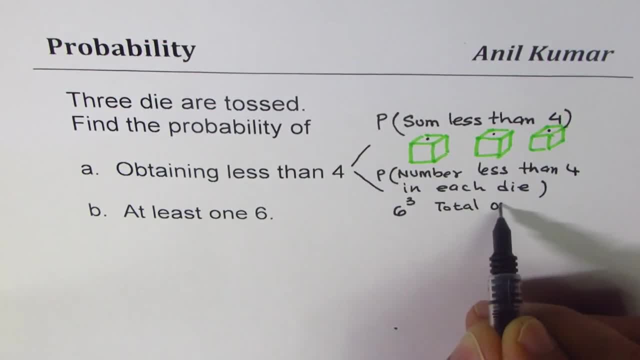 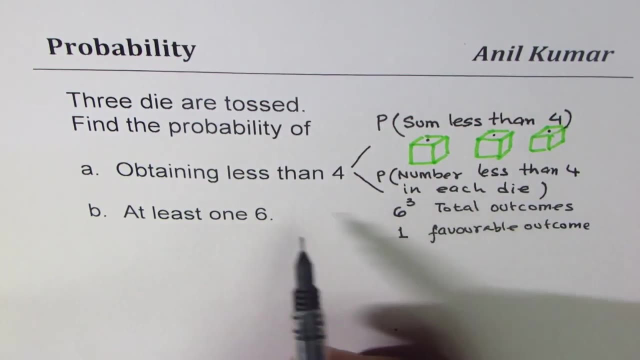 three is total outcomes right and there's only one favorable outcome and therefore the probability of getting less than four as a sum as a sum will be one out of six cube perfect right now. the second one here is number less than four in each die. now there are six numbers in each. so if we take up individually, number getting less. 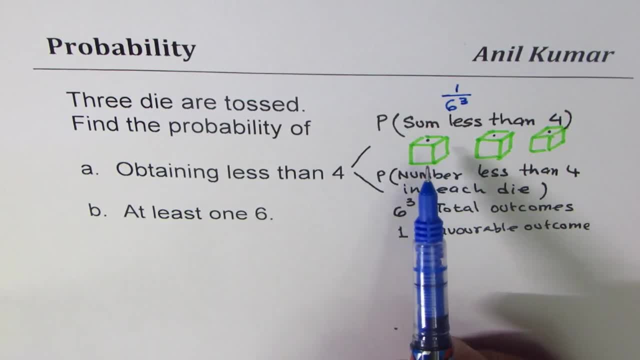 than four means one, two and three, not five six, not four, five six. so the probability is half half and half. so the probability is half half and half. so the probability is half half and half. So for the second option it will be half cube right, or 1 over 8.. 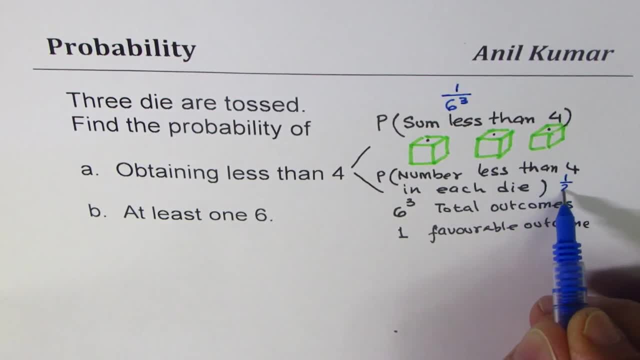 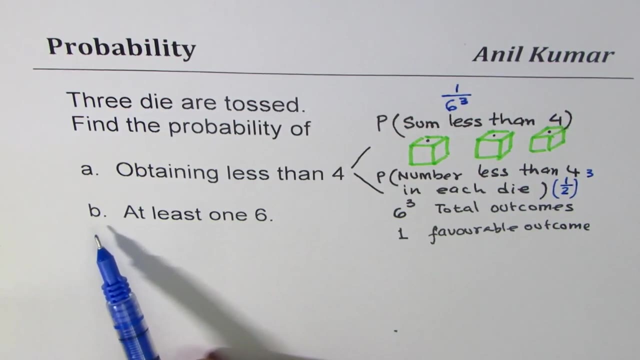 So for the second option, it will be 1 over 2 whole cube. So that is how you could answer it. But I think this question, Part A, is more related with Part B, And what I've done here is I've extended even Part B to make it more interesting. 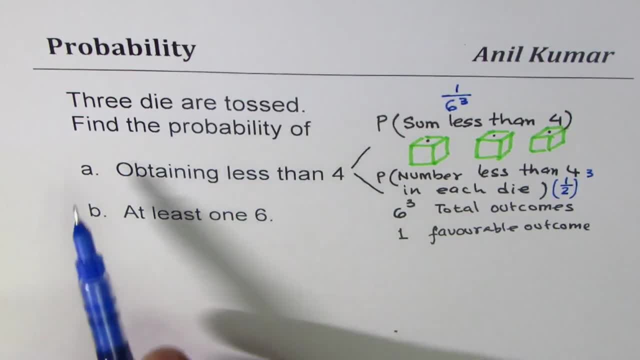 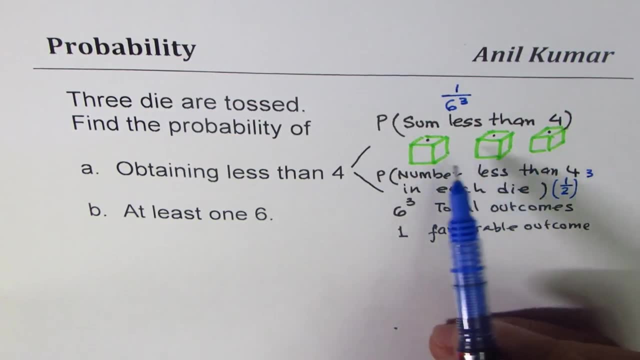 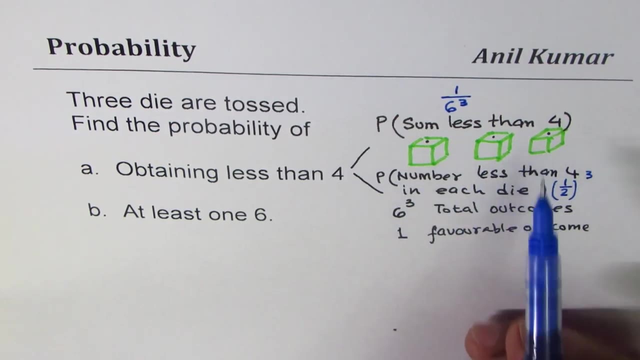 So Part B is three die are tossed find the probability of at least one 6.. So out of three die we get at least six in one of them. That means we could get six in one, we could get six in two, we could get six in three of them. 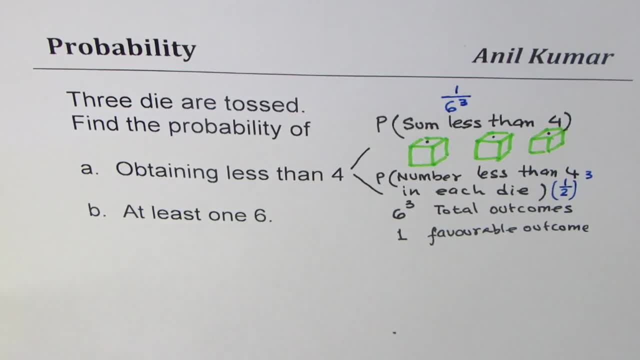 So if you look into cases, there will be so many cases. So what can we think about it? We can think about probability of not getting six right. So let's talk about probability of, not, not six- Let me write it, not six. 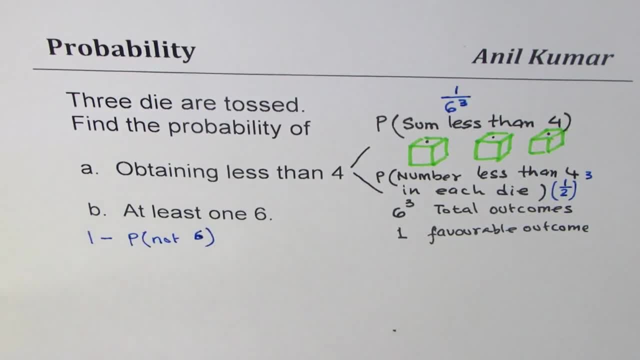 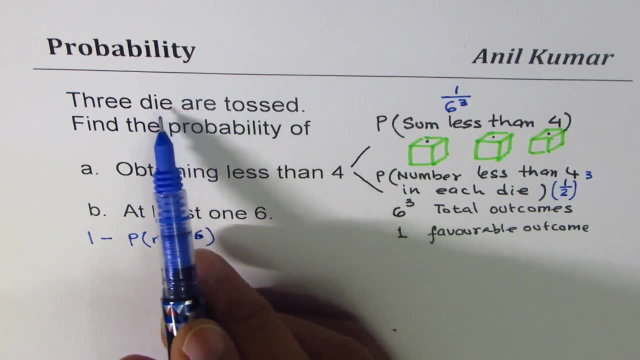 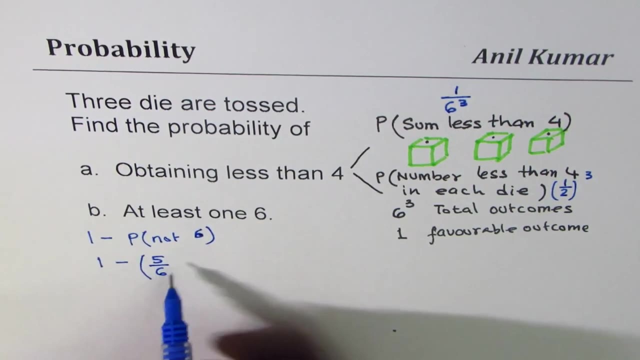 So at least one, 6 will be one, minus probability of not six. Is that okay? Since there are three dies, right, since there are three dies, it will be 1 over 5 over 6. whole cube: 1 over 5 over 6.. 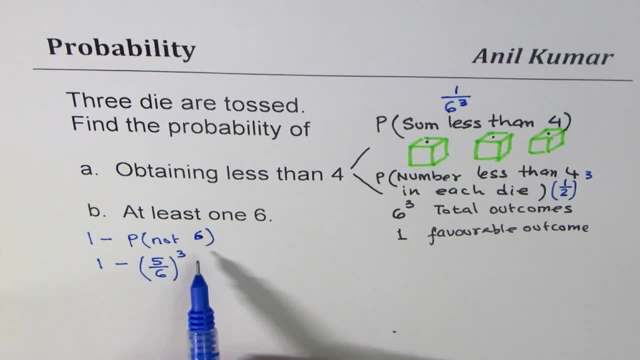 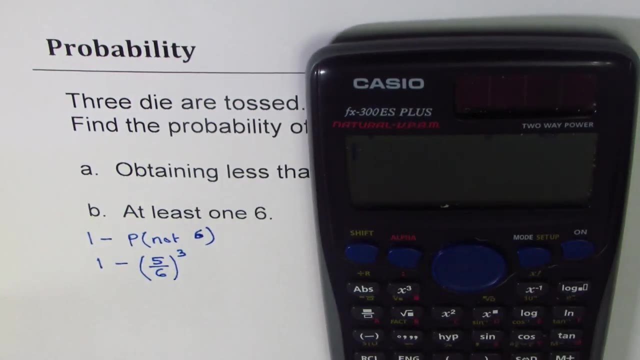 Because there's one 6 and other five numbers are different. So not getting six means getting all other numbers, Is that okay? So the probability is 1 minus 5 over 6 whole cube, which you could calculate, And that is 1 minus 5 divided by 6 whole cube. 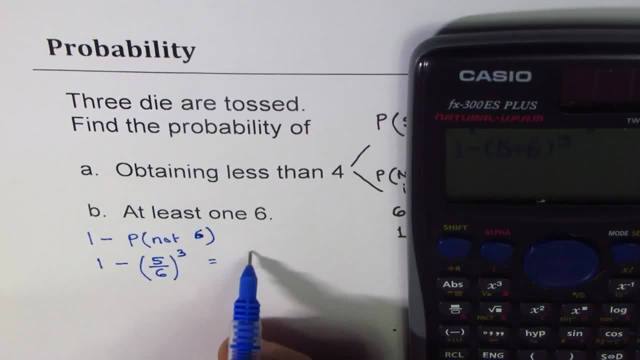 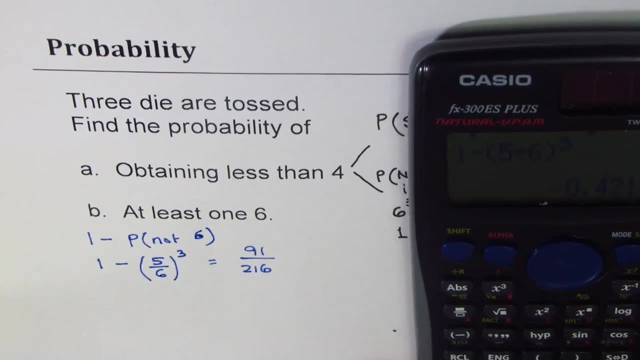 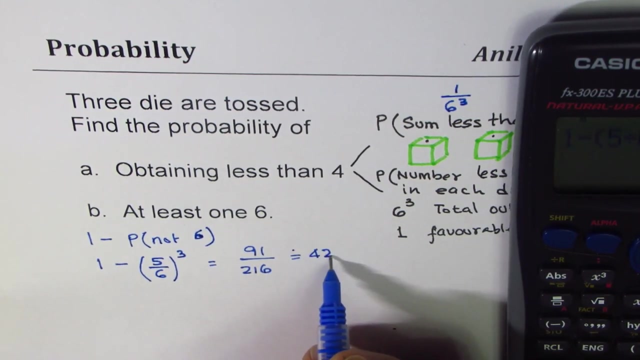 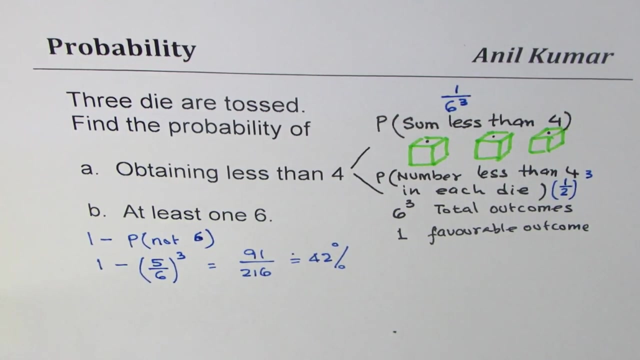 And that gives you 91 over 216.. All right, So you'll convert to decimals approximately 42%. Okay, So the probability of getting at least one 6 is not really very high. You can see it's 42%. 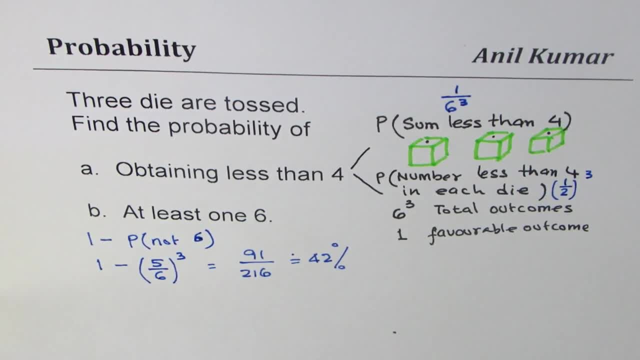 It looks as if when we throw three dies, we may lose, We may get, so it's slightly less than 50% right? So that is how you could answer part B, at least one 6.. And that brings to a very interesting question.